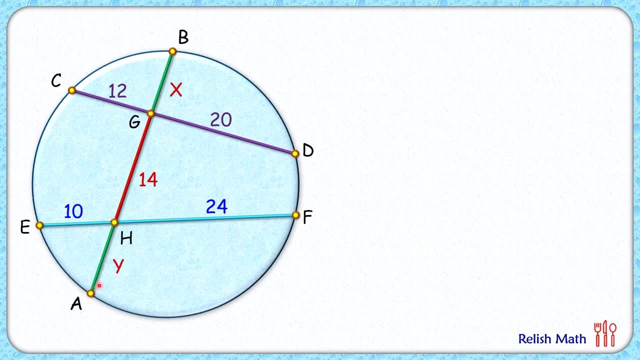 is X cm and HA is Y cm. So here if we look at the chord CD and chord BA Now both the chords, they are intersecting at point G. So applying intersecting chord theorem or power of point theorem, we get: CG times DG is equals to BG times AG. So here, putting the values of CG and DG as, 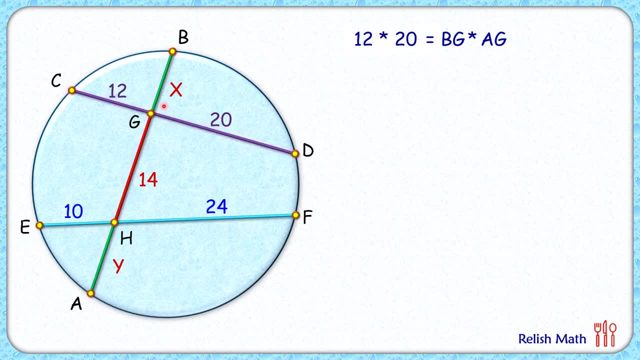 12 and 20.. BG length is X and AG BG length is 14 plus Y. So this is X times of 14 plus Y. Here, solving it, LHS will be 240 and RHS that will be 14X plus X times of Y. Now here, looking at this figure again, we have got chord. 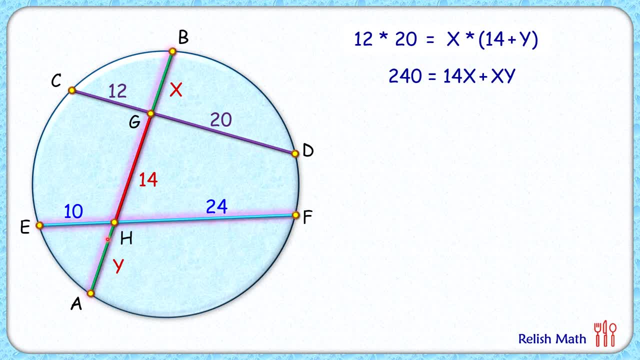 EF is there, which is intersecting with chord BA again. So applying intersecting chord theorem, we get EH times of FH. that's equals to BH times of AH. Now putting the values here, EH is 10 and FH is 24.. AH, that is Y and BH. BH is 14 plus X. 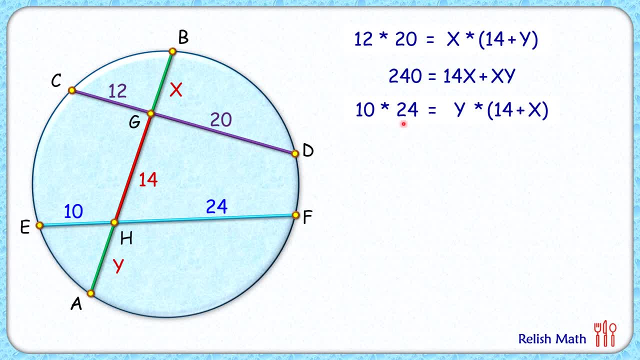 So putting these values here, Now solving it, LHS will become 240 and RHS is 14 Y plus X times of Y. So we have got two equations, two variables. Let's copy down this first equation down below. And now, subtracting these two equations, LHS will become 0. And RHS will become 14 times X. 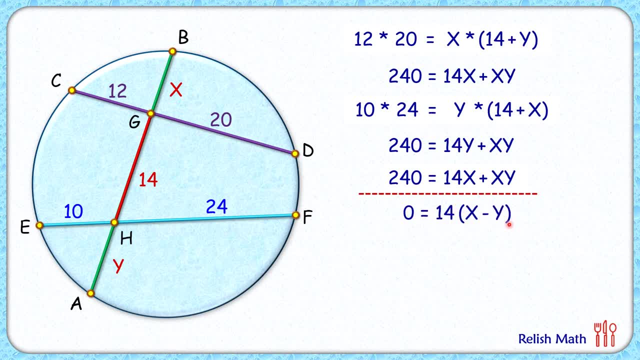 of x minus y. now here RHS will be 0 if, and only if, x is equals to y. so we solving this. we are getting x is equals to y. putting this here now, in the first equation, it will replace y with x. so basically this term will become x square. so the first equation, writing it: 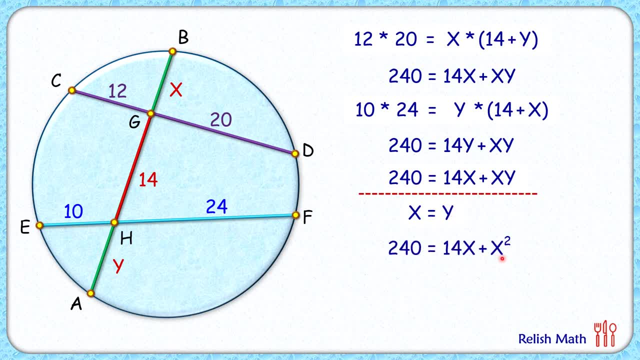 again by replacing y with x, will get this equation. let's take everything on one side, so we will get a quadratic in terms of x. now here, solving this by factorizing the middle term, so splitting the middle term as plus 24 and minus 10, so we will get x plus 24 times.